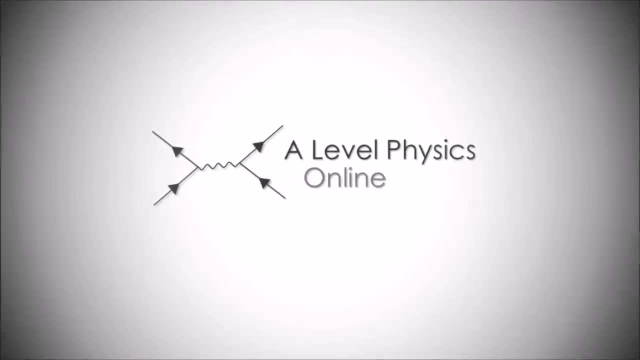 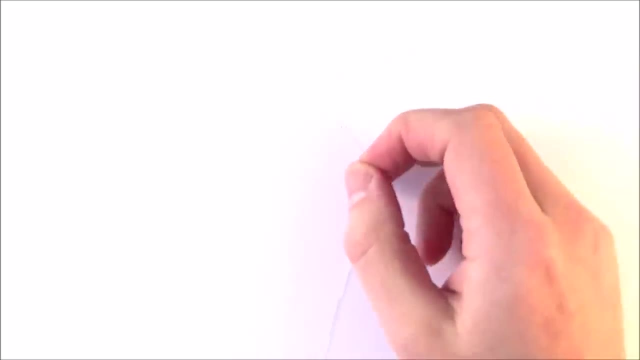 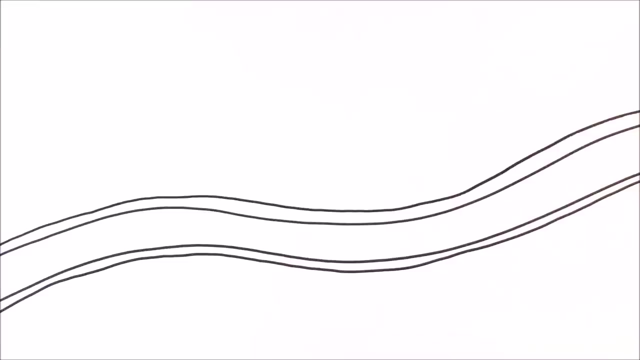 In the last video we looked at total internal reflection and how this works with optical fibres. I'd just like to explain that in a bit more detail and look at the different sorts of optical fibres and some of the problems that we can overcome with them. 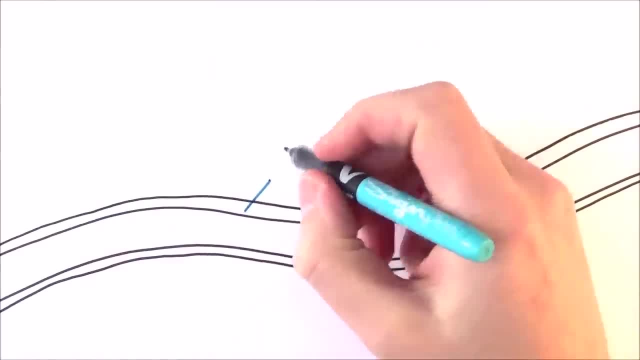 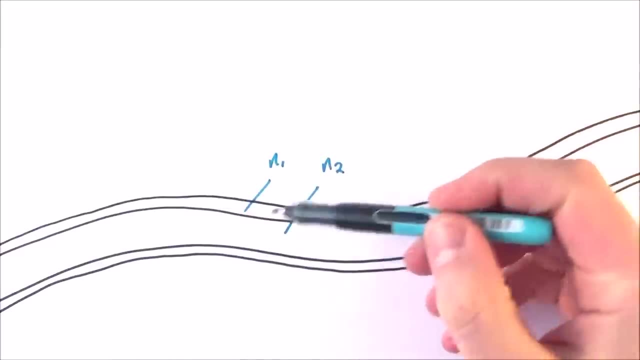 This is a zoomed in view of an optical fibre, and what we might find is that there are two sorts of material inside it and each of these materials has a different refractive index and therefore there's a step change in their indexes. We call this a step index: optical. 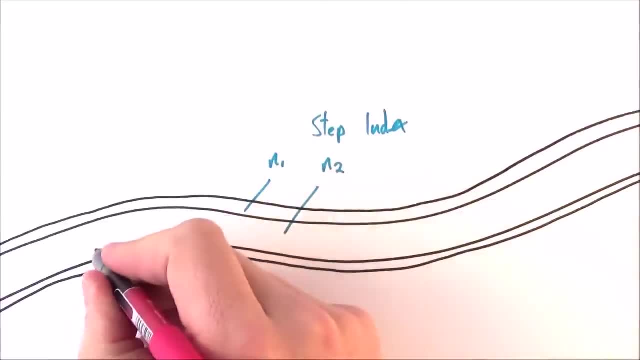 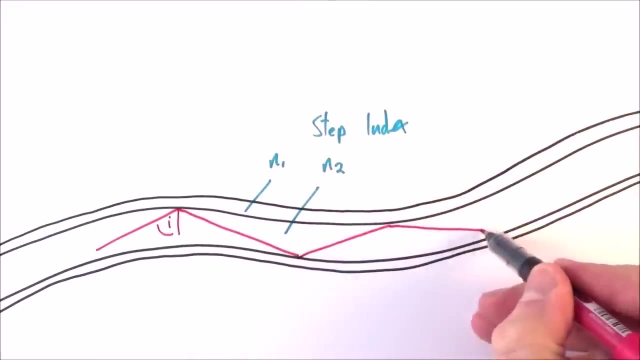 fibre. provided that a ray of light hits the boundary where the angle of incidence is larger than the critical angle, then what we get is total internal reflection. Now, I'm just going to be a bit hasty in my drawings here, but what we have is provided. 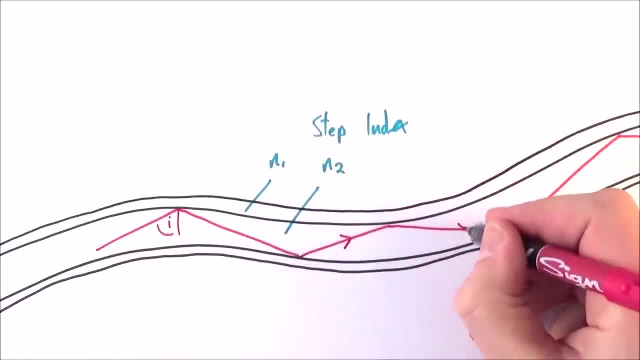 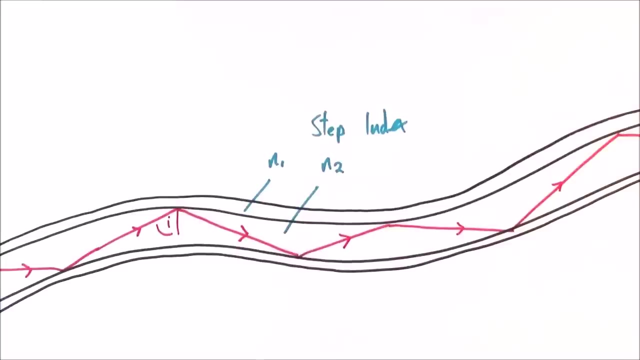 that critical angle isn't exceeded. the ray of light passes all the way along that, and this is how we can use total internal reflection to send light or some other kind of electromagnetic radiation, along an optical fibre. One of the problems, though, is that if we have bits of light that maybe take a different 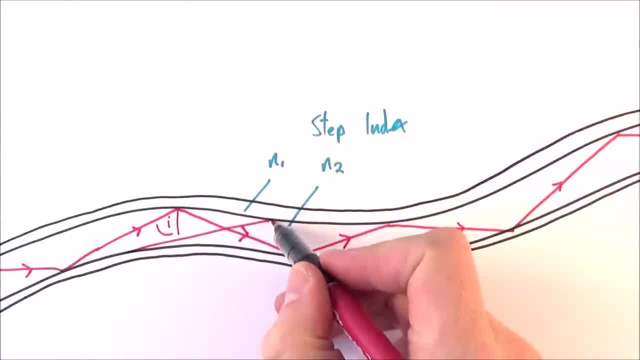 path. perhaps we have another ray of light that is moving like this. what we might see is that, because it's bouncing off different parts of the optical fibre, by the time it gets to the end it actually takes a different length, And what we have then is a problem in the signal. Now, in the olden days we used to use 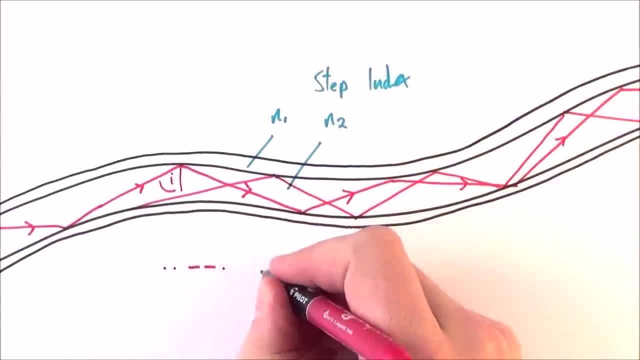 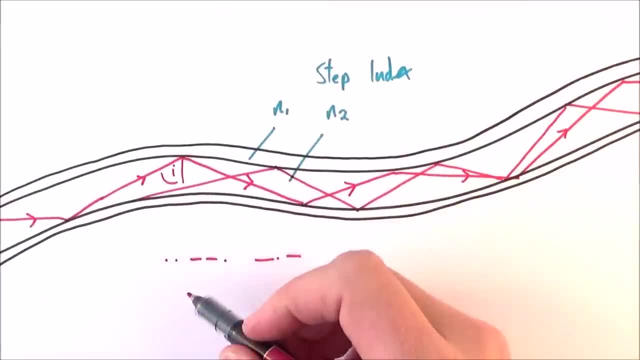 Morse code, where we had a series of dots and dashes and we could send different letters along. Now, optical fibres work in the same way, but this time, rather than having dots and dashes, we have a light source or some kind of radiation, which is either on or off. 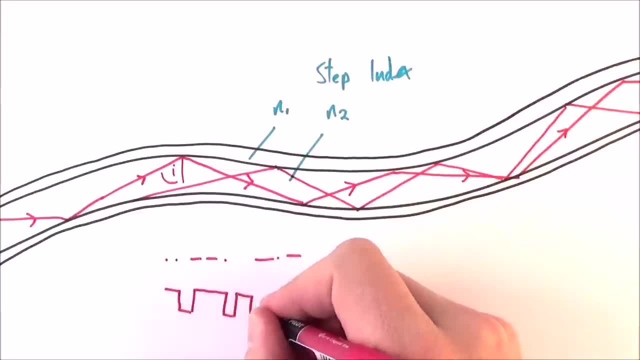 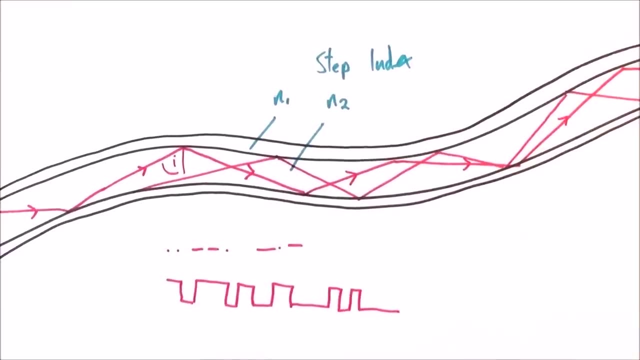 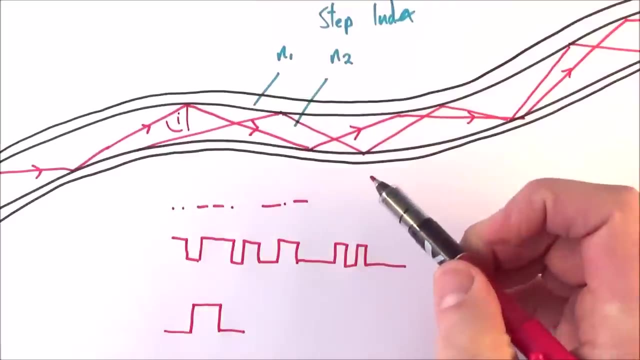 And what we might start with is a signal a bit like this, and what we can do is very quickly have that light actually turning on and off, and this sends a signal along the optical fibre. Now the problem with having what we call modal dispersion is that we might start with a 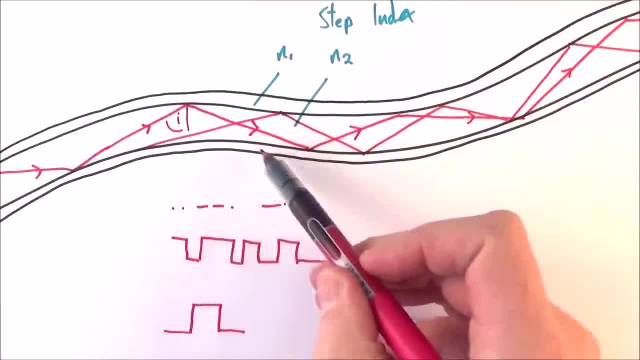 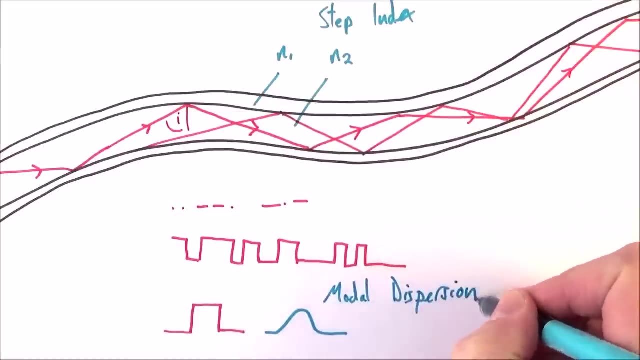 signal which is very clearly off or on, and when that light goes along, some of the light takes along the path and what we end up getting is, rather than a sharp signal, we get something that looks a bit like that, and that is what we call the modal dispersion. 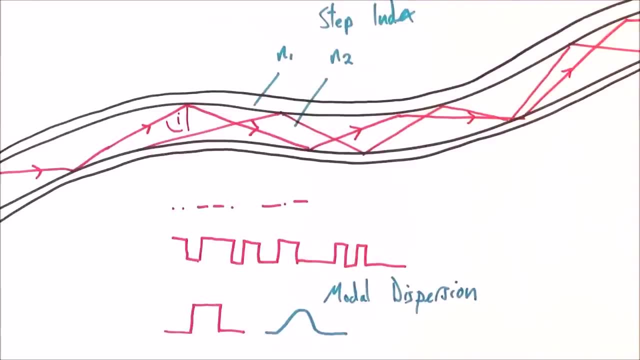 Now, luckily, by using digital signals rather than analogue signals, we have a nice bit of light that strained out. we can still tell roughly if that's on or off. so what we can do then is we can put this through a filter and then we can say: well, at this time here it was maybe off, and at another time it was. 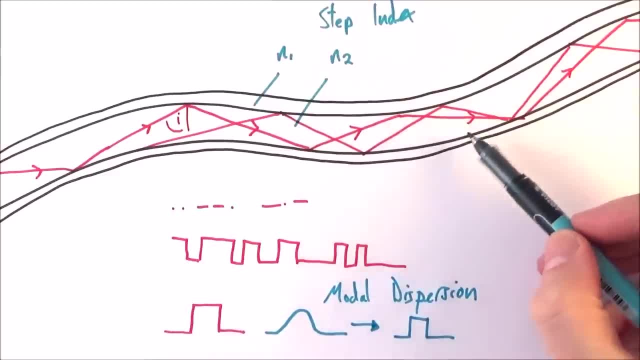 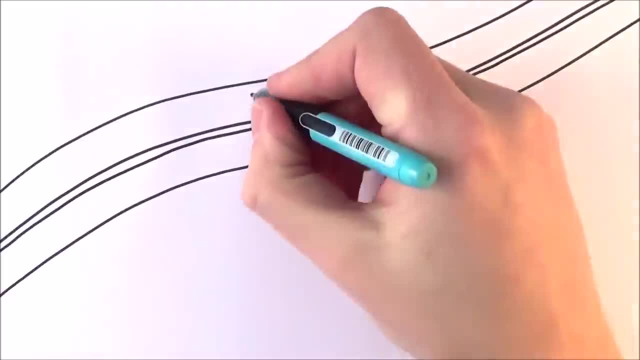 on and this means, although there might be some the signal might not be getting through perfectly, we can apply a filter and we can get back to the original signal. This is another solution. what we can have is material, where we have again the two different refractive indexes. so maybe 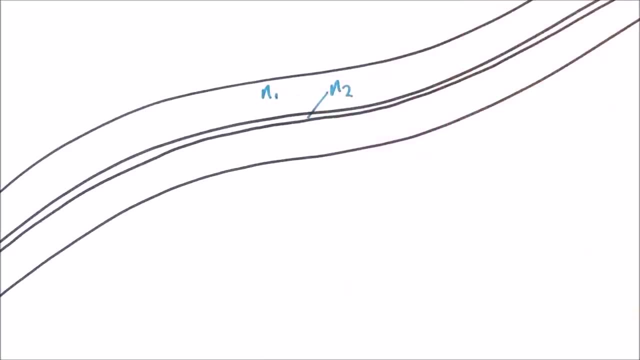 n1 in the outer layer and n2 on the inner, but this time the inner core is a lot narrower. so what this means is that the rays of light moving down it, they have less chance to have a different path difference and therefore every ray of light moving along in what we call a monomode optical 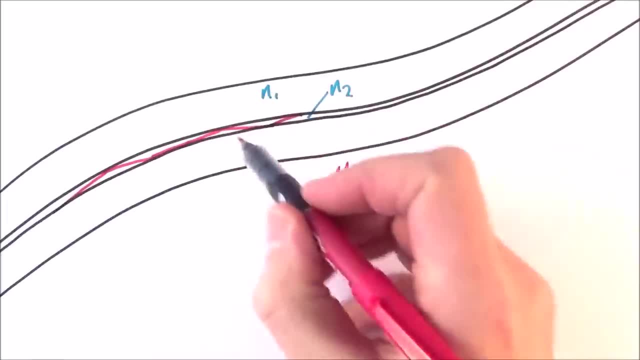 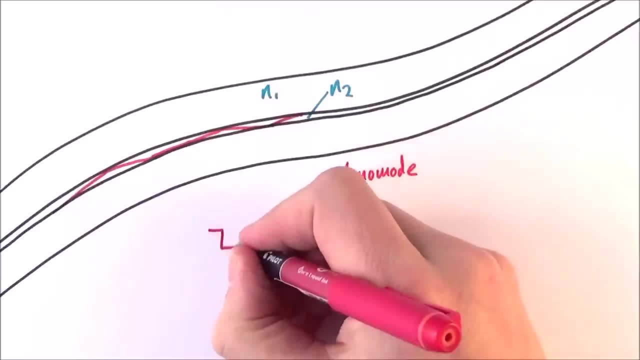 fiber, every ray of light doesn't have the chance to spread out and take a different path length and again, this gives us a high quality digital signal at the other end. so what might go in as a series of you know ones and zeros, or ons and offs, we get out at the other end. 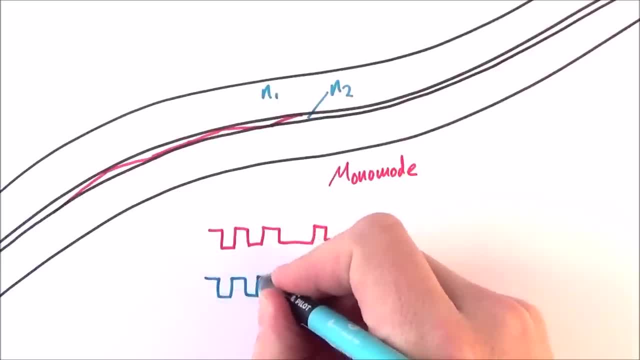 very close to that original signal and this means that we can send data very, very quickly over long distances. we don't need to have lots of boosting stations along the way, so we can send very long cables and we don't need to have the expensive equipment at the other end to sort of. 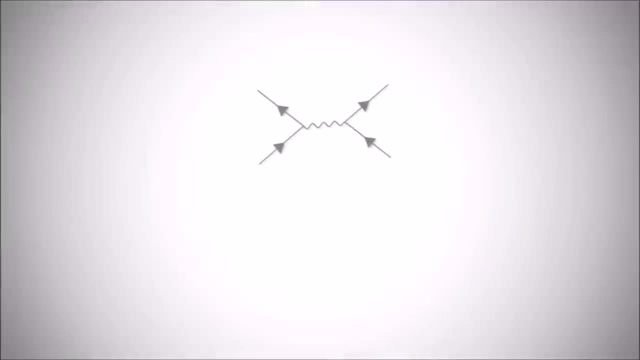 try and filter out the original signal. So this is kind of a very basic thing in this particular case and I'm not really sure what that's really about. so the information that I am trying to provide in this video at this point is very important, because I don't want to go through the whole thing, but it is very important to have some kind of understanding of this kind of information, and this is why I will be doing this in this video, because it is necessary to know what theige is and what the range of, what the range of the range of light is, and this is kind of what the ionized red is. a lot of things Now, So